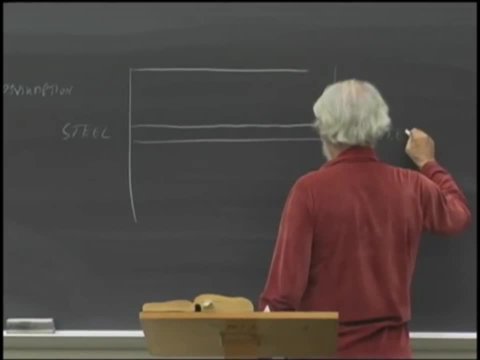 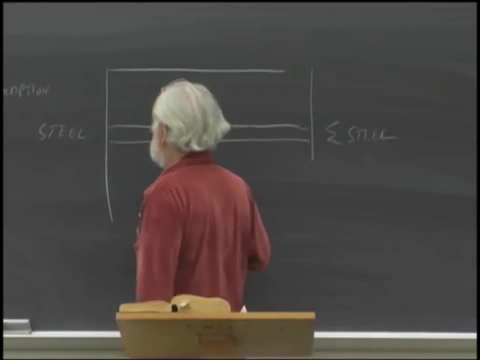 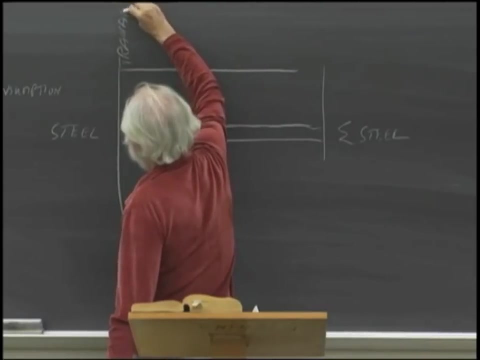 the total amount of steel produced. You add up all of the steel- Now let's say it's just tons, physical tons at the moment- And then you ask the question: how much steel goes into a sector called transport equipment? Okay, so you have a sector here. 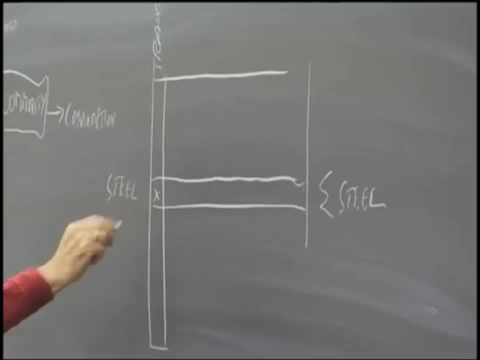 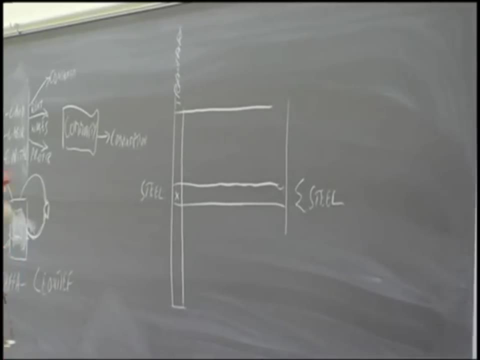 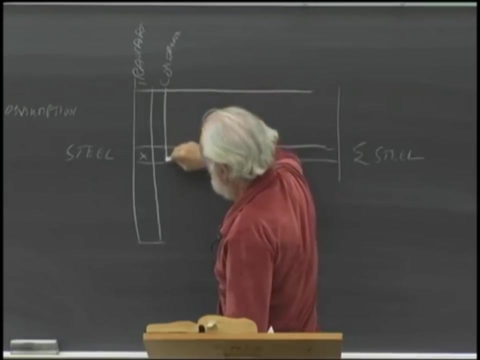 And you enter a number here of some kind, which is the amount of steel that needs to go into the transport sector. Then you say the amount of steel that needs to go into construction, Okay, And you end up with another number. And so you keep on going over across all of the sectors in the economy, over here. 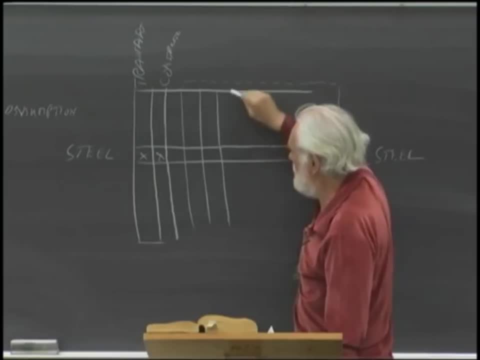 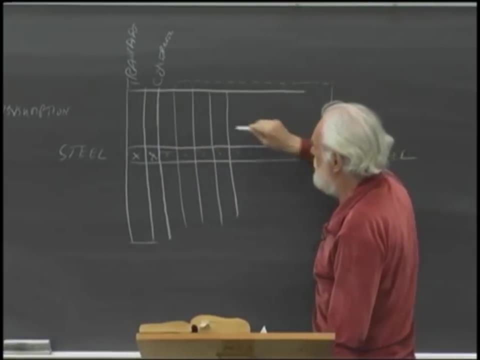 and you end up with something like this And you add up all of these steel going to all of these. So this is where the steel is going Now. one of these will be steel. How much steel do you need? How much steel do you need to produce steel? 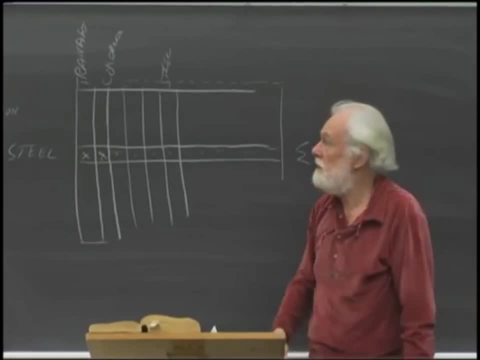 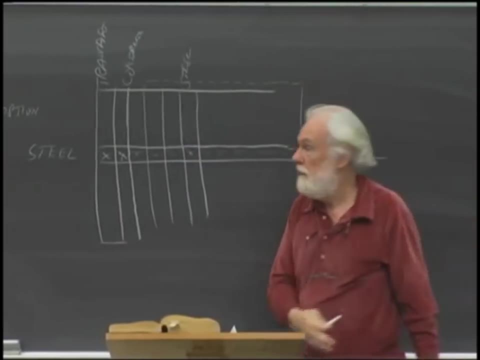 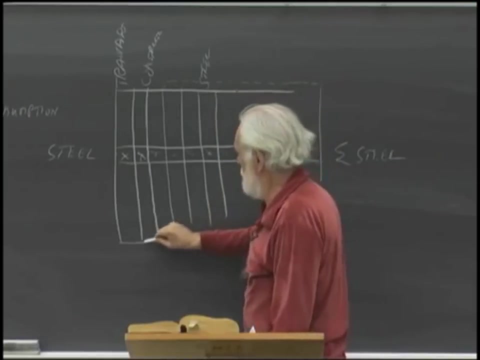 And sometimes you do need steel, and this is going to come up in here, So there'll be an entry here. Some of these spots will be empty. No steel is needed to produce this, But when you take steel here, then actually, as you take all of the sectors over here, 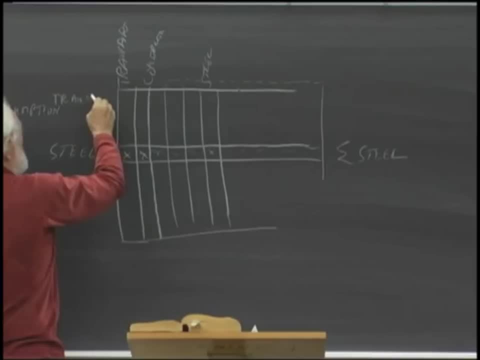 so you'll have transport here and you say, well, how much transport do you need to produce steel, How much construction do you need, How much iron ore do you need? And you end up, so you end up, with a matrix of this kind. 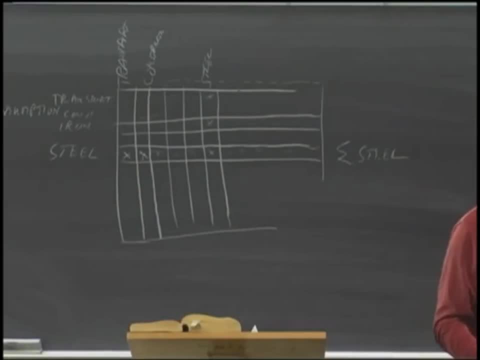 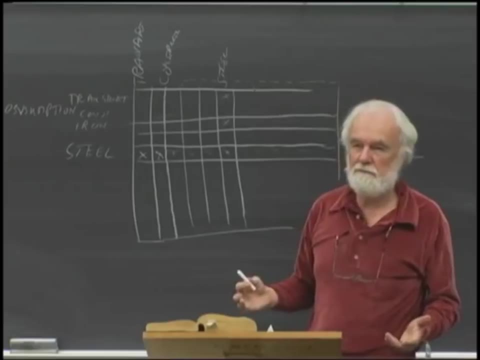 Right Now, this is an input-output matrix, And what's very interesting about this is, let's suppose you decided you wanted to expand steel production, Okay, And you said: all right, our aim is to increase the output of steel. 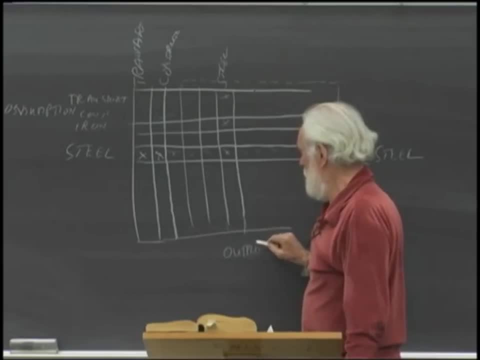 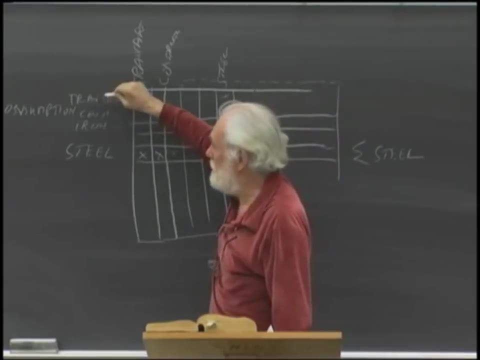 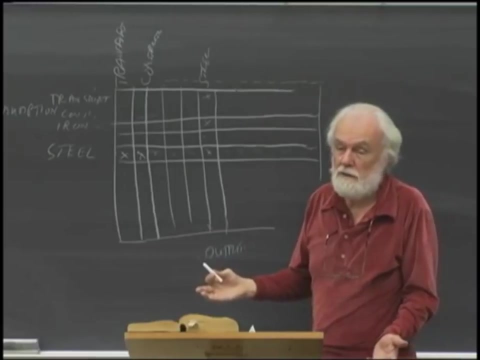 This is the, And we want to increase this. Well, we're going to have to increase all of these inputs by so much. Where it's empty, you don't have to do anything. But if you're doing central planning, you kind of say: all right, we want to double steel production in five years. 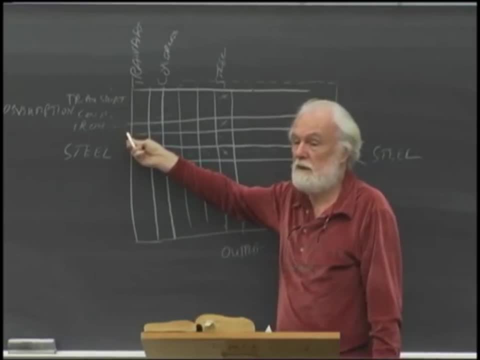 How much more iron ore do we need? How much more coal do we need? How much energy, extra energy do we need? And we can actually use this and we end up with a set of codes, coefficients here, which are mathematical coefficients. 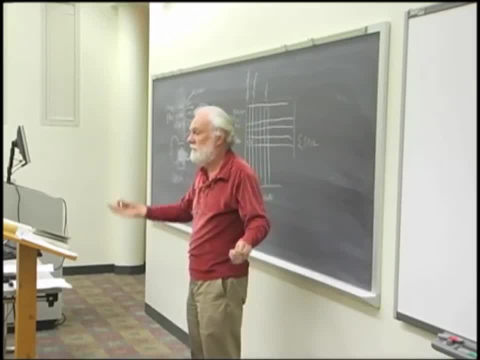 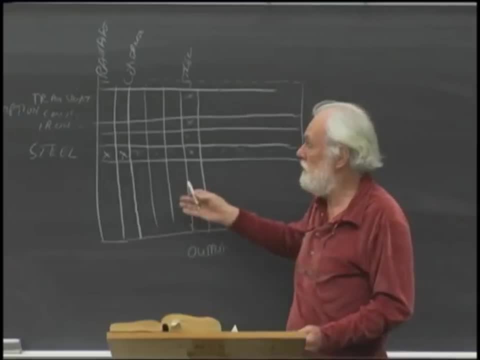 and we can then simply calculate how much of anything we particularly need, if we want to double the output of steel, or we want to double the output of automobiles, or something like that. So this is what we call an input-output table, And it can be used in this. 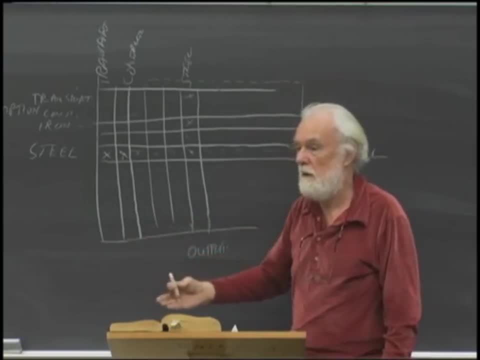 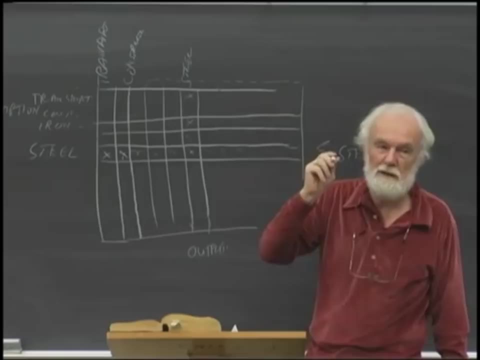 And this is what is really meant by the production of commodities, by means of commodities That you can only produce steel by taking a whole bunch of commodities and putting it into steel production. You can only create, You can only produce, You can only produce. 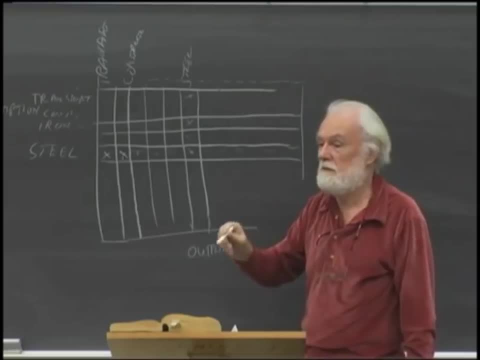 You can only produce transport equipment if you take a lot of commodities and put it into transport equipment. So, Leontes, This takes off from Marx's matrix as well as you can see what the connection is, So input-output. And this, by the way, is now: 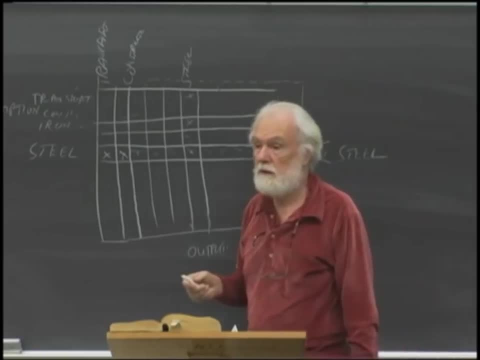 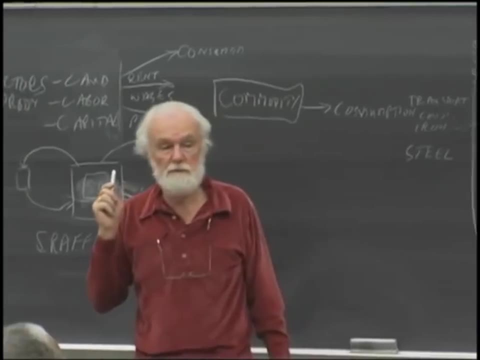 is still the framework of national accounting And you could use this for planning all sorts of things, like it was being used at the end of the 1960s by several people, for instance, who were interested in the question. let's suppose you halved. 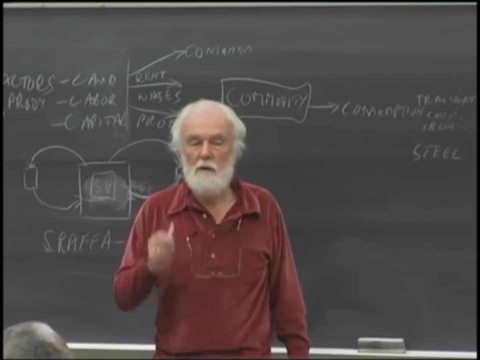 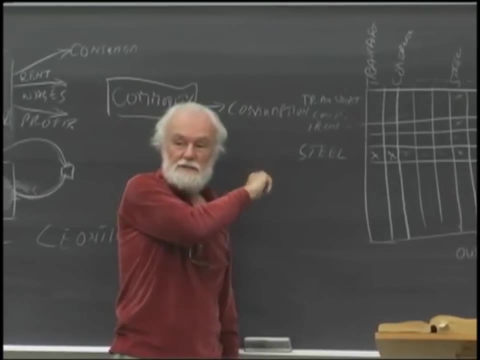 the defence budget, right, What would be the impact? So you could find how much steel would be reduced, et cetera, et cetera, et cetera, by halving the defence budget. What you could then do is to say: 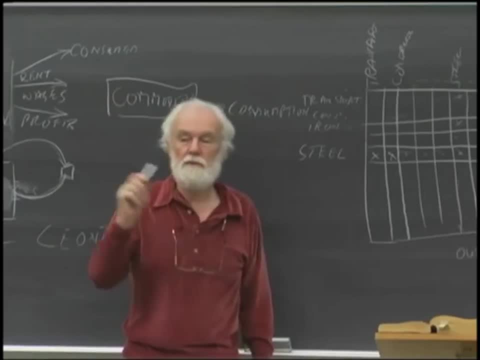 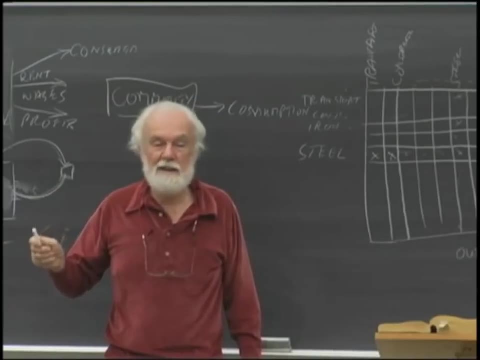 all right, let's suppose we halve the defence budget and we double the budget for hospitals and universities. Yay, that's a good idea, All right, And then you could see what would mop up: all of the resources which have been. 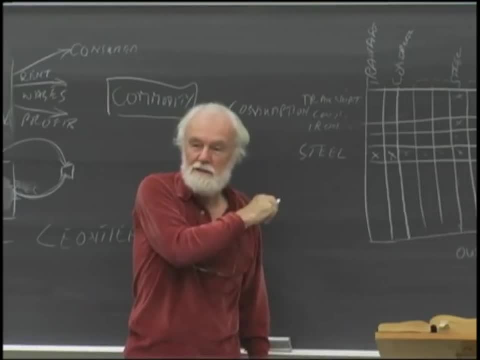 lost by closing down the steel or closing down the defence industries or seriously covering them back. So there's a lot of planning which uses techniques of this kind and it was very heavily used in the 1960s, 1970s. Now, since then, of course,